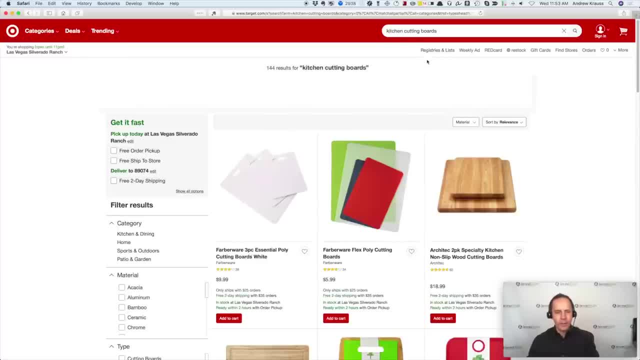 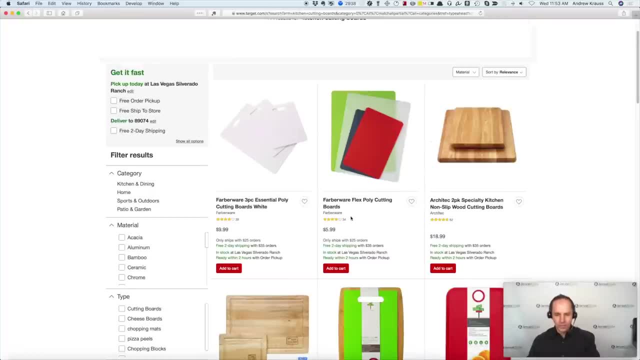 I'm just looking for any random company to call, but a company that's actually in a major retailer you want to be in. So I typed in kitchen cutting board in target and you can see here this company is this farbware right? And then this company is selling these. that's farbware. This company is. 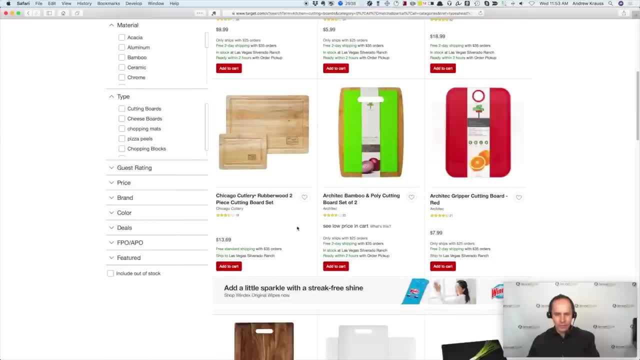 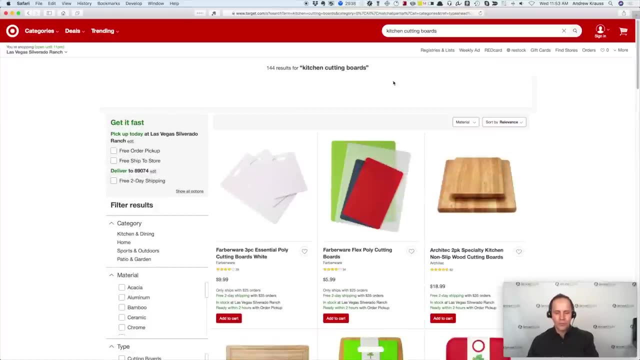 architect, And then you see some more Chicago cutlery, architect, architect. So I'm not telling you to contact these companies, guys, You need to do this yourself. Find a random company, because if all you are calling the same company, that's not going to work well, You'll be like what's going on? 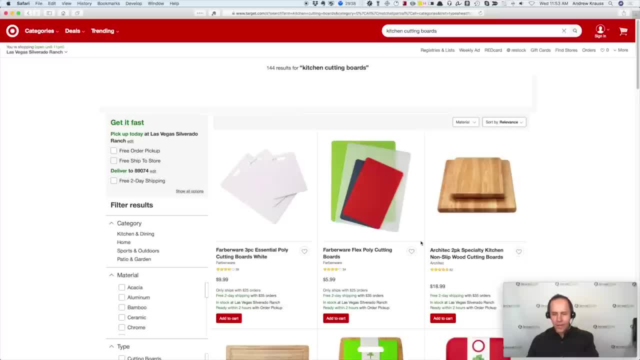 here. So so we got the name of the company. It's right here, This one, the name of the company, is farbware and this one is architect. So let's do architect first. So I'm going to do is I'm going to. 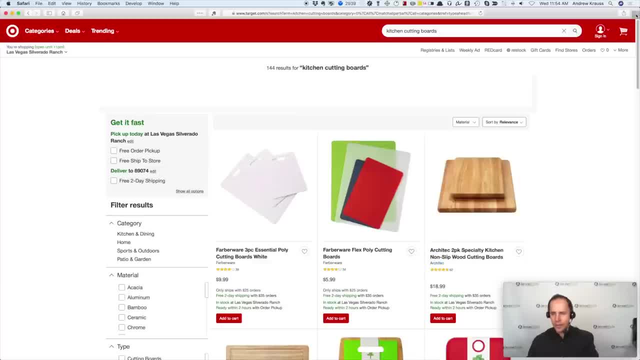 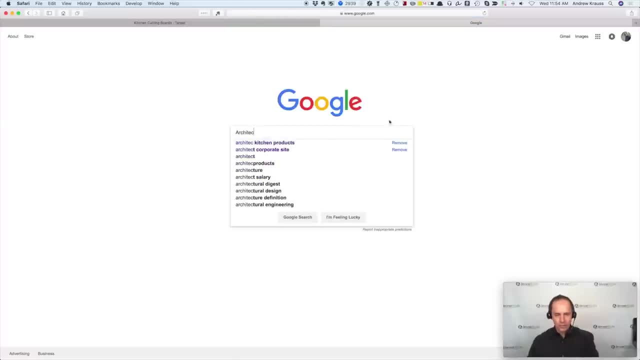 copy the name of that company. I'm going to open up a new tab in my browser- Not hard to do, right? And I'm going to search architect. Now it's a kitchen product, right, I'm going to type architect- kitchen products because it's a, it's a cutting board, So I'm 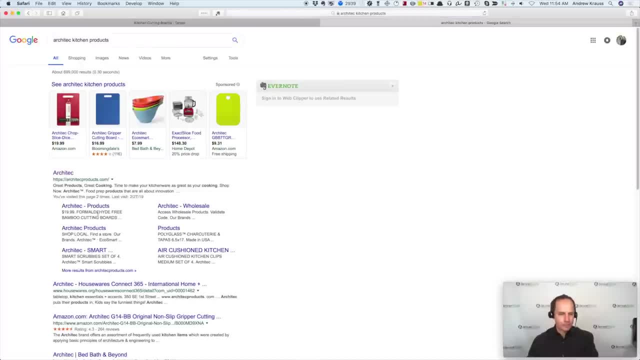 going to type, because what we're looking for is the company website. Okay, So right here, we found them really easy. I didn't just type in architect, because I did that before and you get all these architects right. That's doing buildings and things, But I type in architect space kitchen. 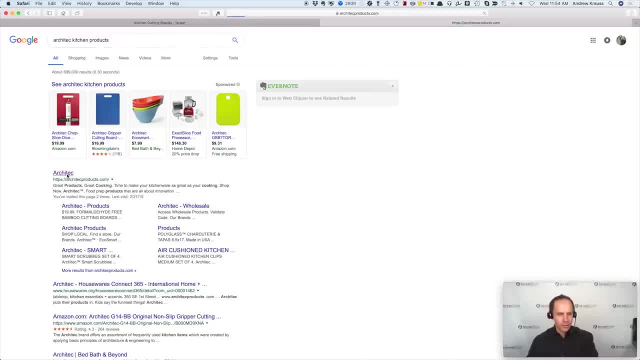 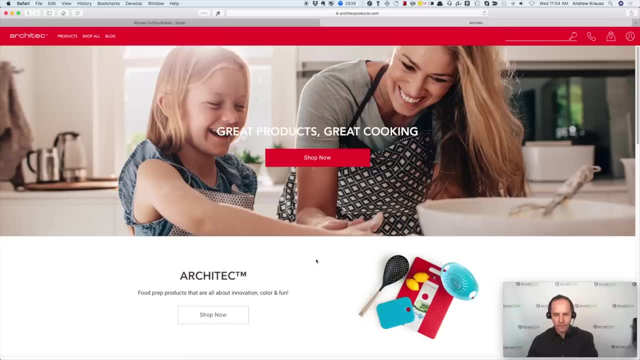 space product, And it's right there. architect products, And you know it's the company because you can tell by looking at their, their homepage. you know it's okay, It's kitchen products, All right. What I like to do is I like to just jump right down to the bottom, look for a contact us button. 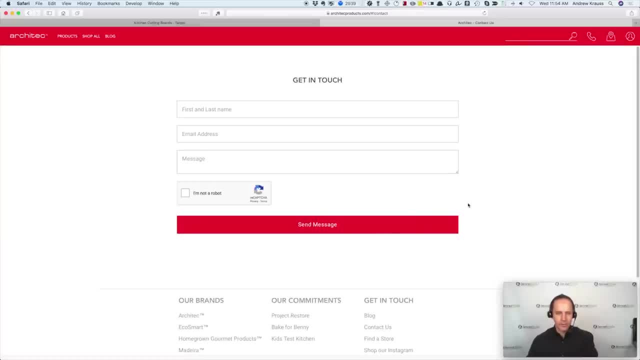 I'm going to do that. I found a button, Oh damn. Okay, Just a form. Well, that sucks. Okay, Let's see if we can find a number here. I'm going to click on this little phone symbol and guess what? 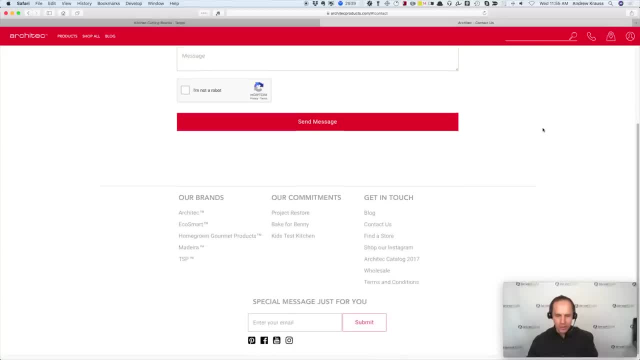 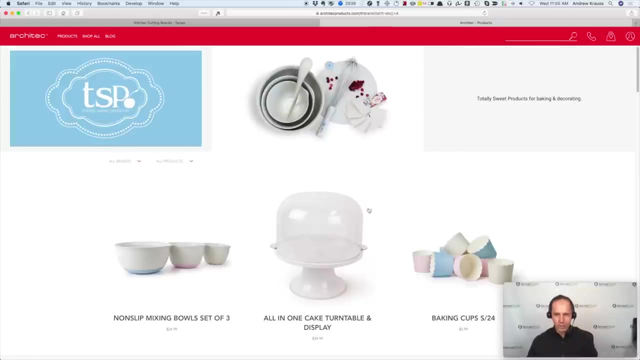 It takes us to the same page, So they're not giving us a phone number, are they? Let's see So all their brands they have: architect, eco, smart, homegrown gourmet products, area Madeira and TSP- Let's click on TSP. Um, didn't take us to another website- has all their. 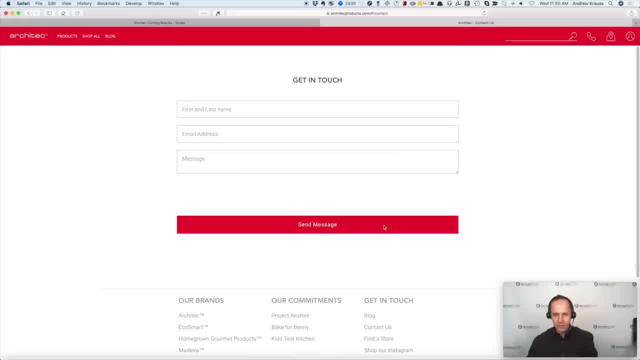 products really, really helpful, but still don't have a click on contact us again. Okay, Just phone number. Now I could Google for this. I could type in architect corporate website. I did that a minute ago. It didn't work, but you could dig up the, the, the a phone number for this company. You. 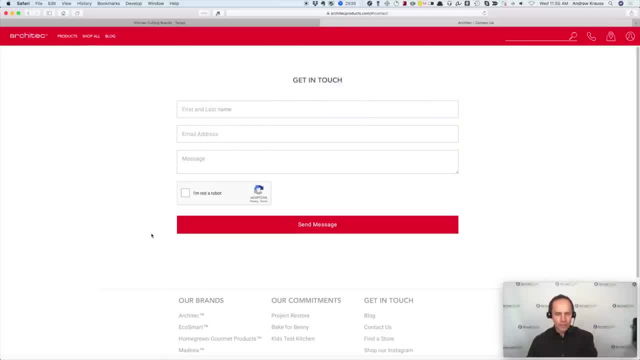 could also drop them an email through this form and say: you know, I I'm looking to see if there's a product that I'm looking to submit. I'm an independent product developer. I'm looking to submit a product to your company, Who would be the right person to contact? You could put your 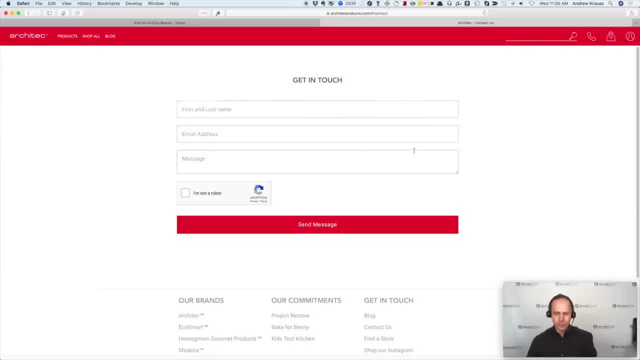 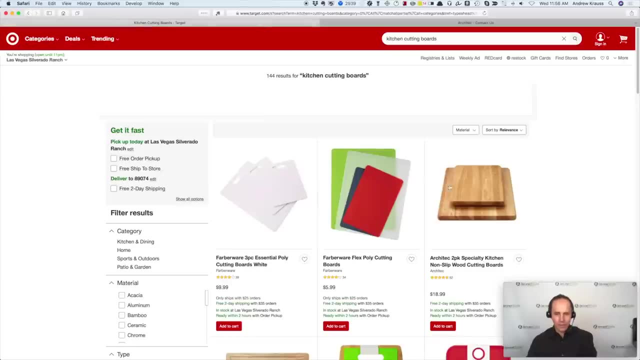 your first name, last name, email and your message in there and send it to them. Okay, Or you could Google a little bit more and you could find their, their corporate website and call their corporate number. So let's do that again with a company I'm more familiar with: Farberware. 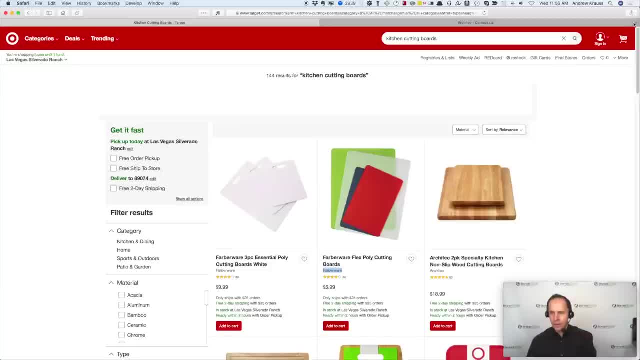 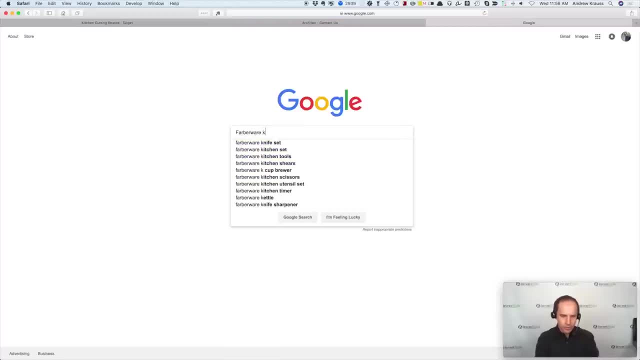 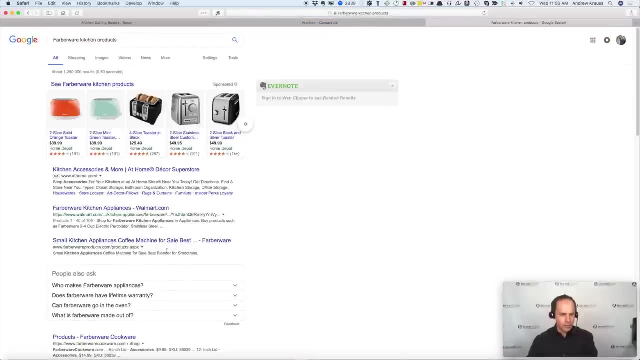 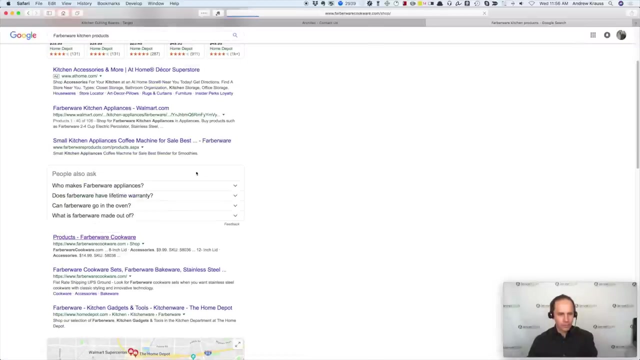 So again, I'm going to copy the name of that company and I'm going to paste it in here. Type in: let's do it again: Farberware, kitchen products- Okay, And let's see Farberware. I see farberwarecookwarecom. These other ones were like Walmart and stuff. See where this takes us. 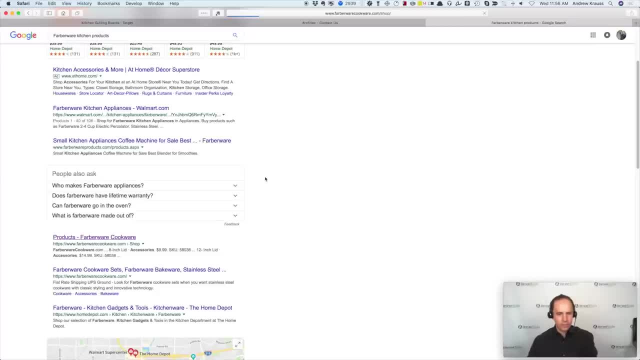 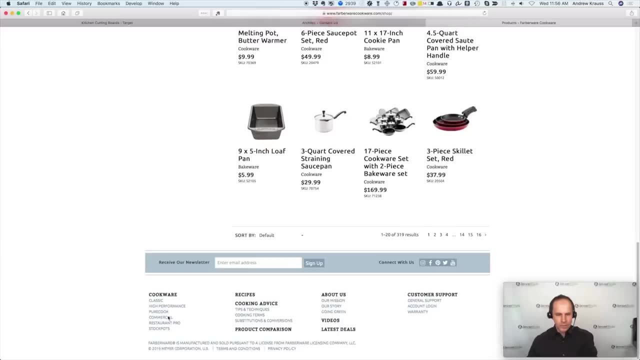 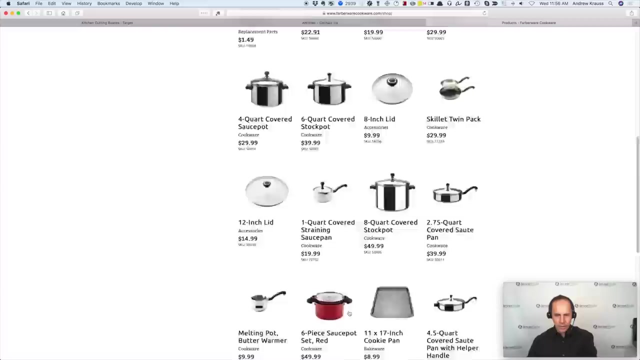 That was awfully slow. Ah buh buh, buh buh. This is more of an ordering website. Let's go down to the bottom. Contact us, Cookware recipes, about us, Sometimes videos. Now you know I came across. 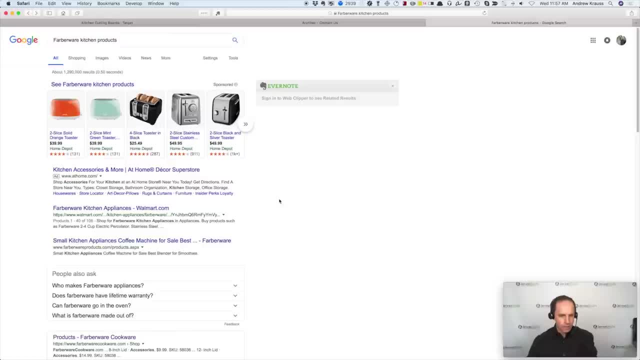 another Farberware site when I searched this before. Let's take a look Instead of doing Farberware kitchen products. you see, this is a perfect example of the same thing. doesn't work all the time. Farberware is a very big company, So we're just going to search, search Farberware. Ah, but that's. 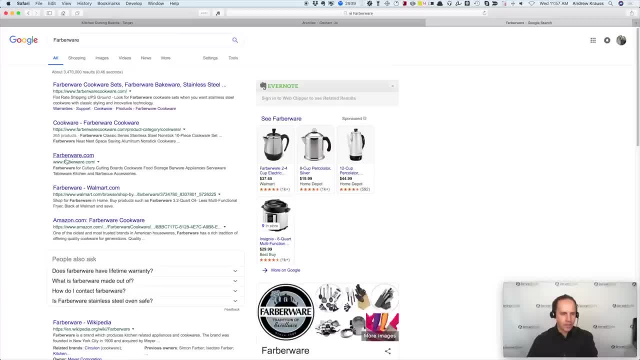 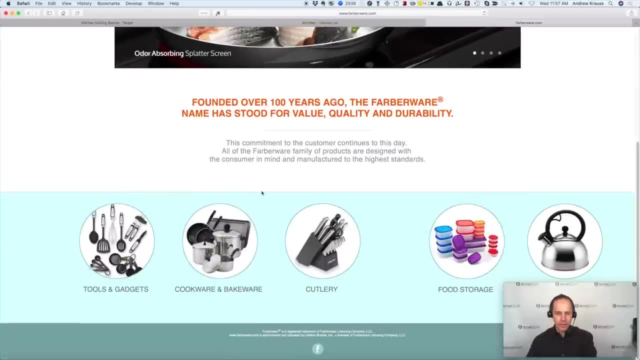 much better. I kind of did this on purpose, guys, But um, and I just see Farberwarecom. You can also just type the company name, com. That's quite often what it is. So I went to their website. Oh, okay, And it's. 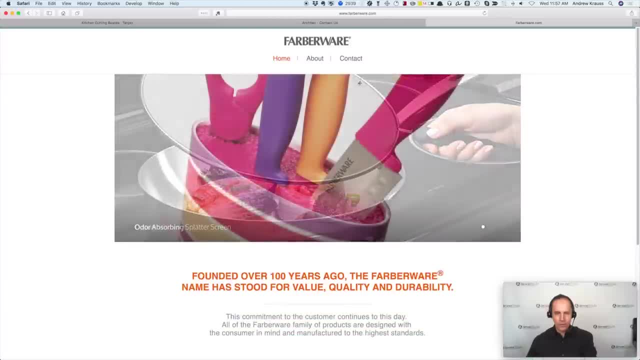 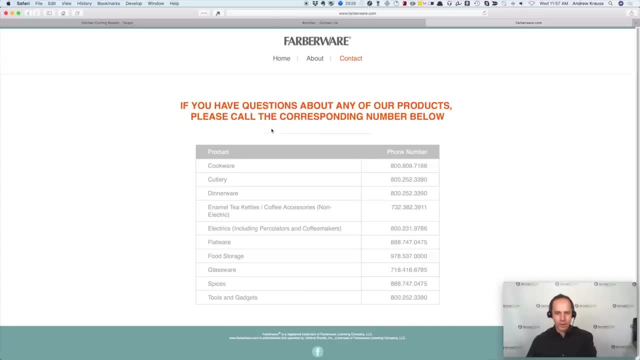 showing you know all their different products. here You can click on and get more info. But right, big as heck, right up there is just contact. Oh, okay, If you have any questions about any of our products, please call these corresponding numbers below. Cookware cutlery: They got different phone. 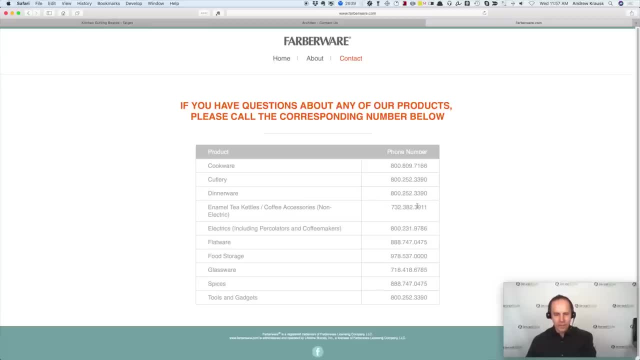 numbers. They're very customer oriented. Now, these are customer numbers. You don't want you don't want to talk to these folks, but that's okay, They you want to talk to them. to help you Contact one of these numbers and then say: you know, I'd like to get a hold of your marketing manager for your 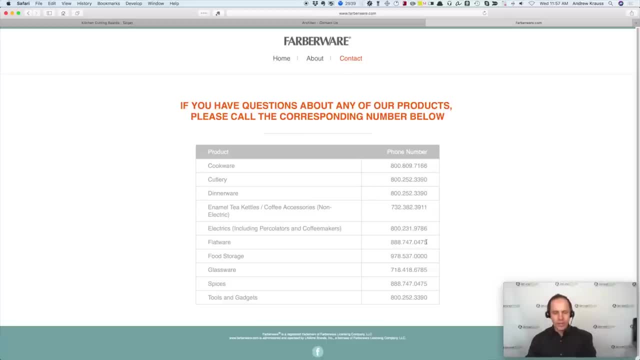 flatware Say I'm not. I'm not a customer, I like your corporate number. You could just say: you know, because the people that pick up these lines, if they're just doing flatware and they're like they're. 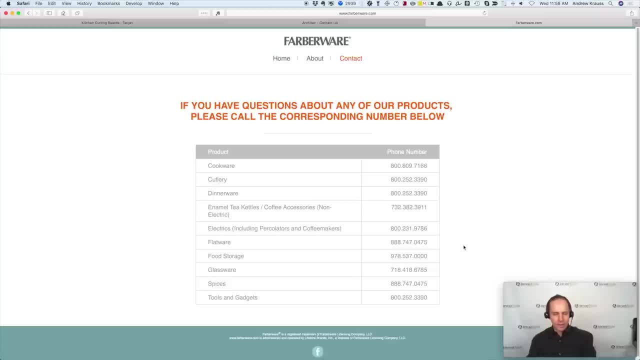 used to helping customers, So say: you know, I'm not a customer, I'm a vendor and I like your corporate number. You could say that, Um, and they'll probably give it to you. They'll give you the corporate number. They don't have it right. 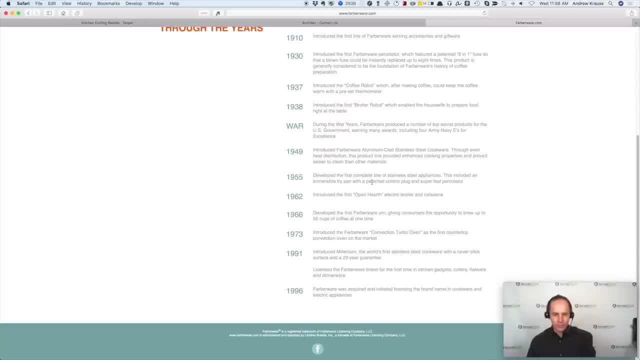 here. You could probably dig around and maybe find it some other way, um, on the internet as well, But anyway. so I don't want people to say, well, I can't get phone numbers, So I just want to give you a. 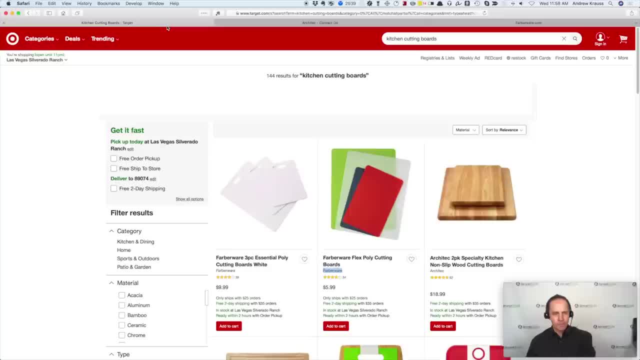 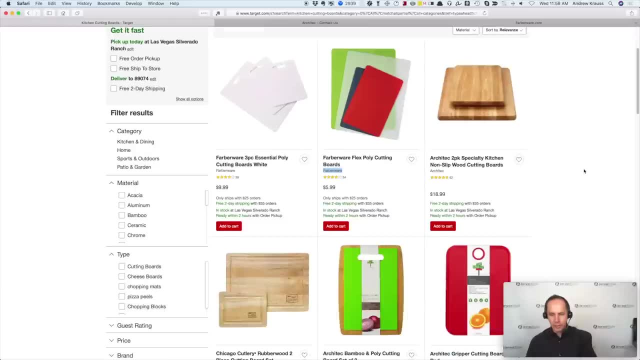 basic, basic overview. And if you do this with a couple of companies on a website like target- don't do cutting boards, do something else, do anything Um- and you can't find a number, Just look at another company, Like if both these two didn't produce a number, you could do Chicago cutlery and do the same thing. 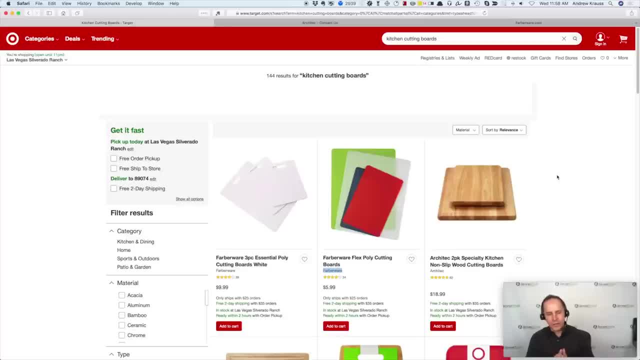 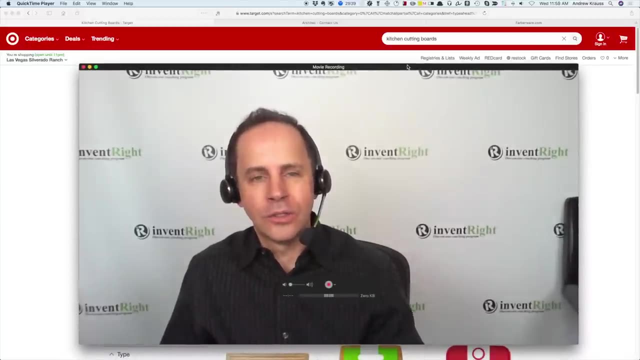 Because the main goal here is for this video is not showing you how to how to search, uh, for companies and phone numbers. The main goal is I want you to call these companies and basically say: are you open to product submissions? and say: can I submit a product to you? That's what I want you to do. I want you to call these. 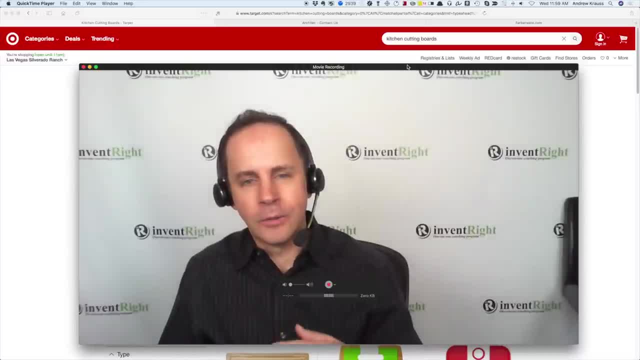 companies and say: I'm a product developer, I develop and license new products And um can I submit a product to your company? What would be the approach? What would be? who should I call? Who should I talk to? 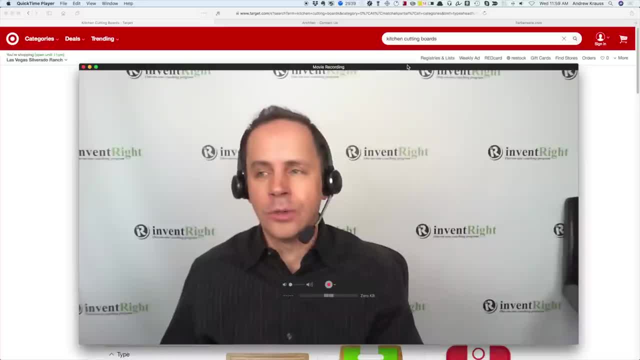 And they may not know. And if they don't say, well, you know how about? uh, your marketing manager handles your flatware, or the hill is your cutting boards, or something like that. So I'm not telling you to call these.